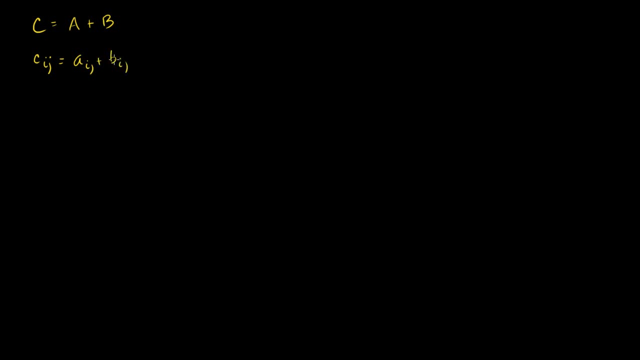 A plus the ij entry in B. That's our definition of matrix addition. You just get the corresponding entry in the same row and column, add them up and you get your entry in the same row and column in your new matrix. It's the sum of the other two. 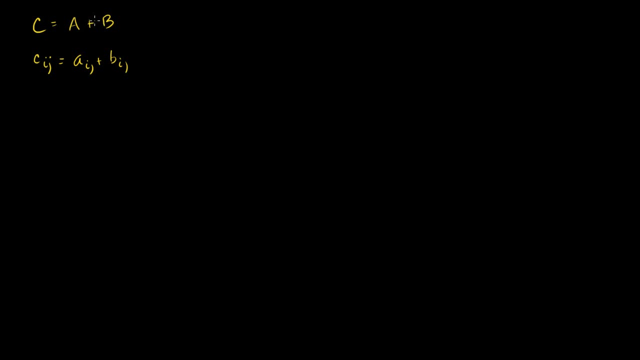 Now let's think a little bit about the transposes of these guys right here. So if A looks like this, I won't draw all of the entries, It takes forever, But each of its entries are ij, just like that. Let's say that A transpose looks like this. 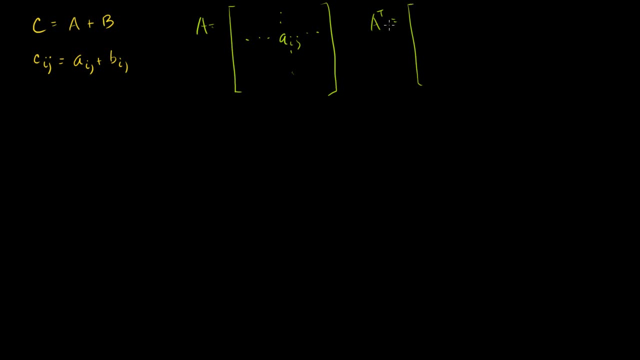 Each of its entries, we would call it. let's say, if you've got that same entry, we're going to call it A prime ij, And these things aren't probably going to be the same. There's some chance they are, but they're probably not going. 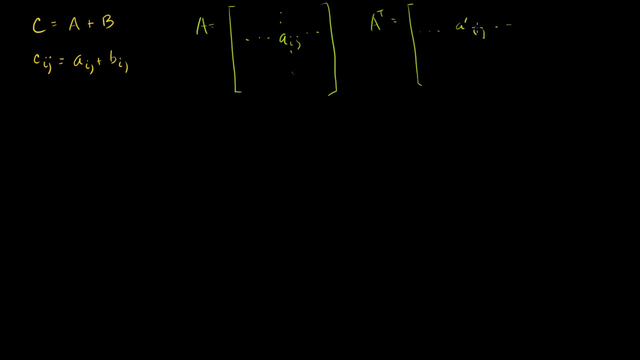 to be the same, But that's its ijth entry in the ith row, jth column in A transpose. Now, The fact that this is the transpose of that means that everything that's in some row and column here is going to be in that column and row over here that the rows and 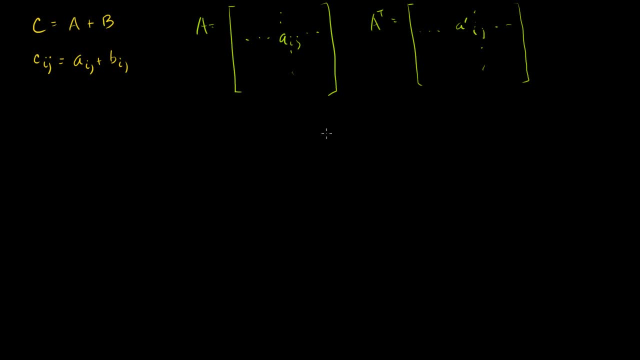 columns get switched, So we know that we could write that A prime ij. we're going to have the same entry that was in Aji- Maybe Aji is over here, So this thing over here, which is in the same position as this one, is going to be. 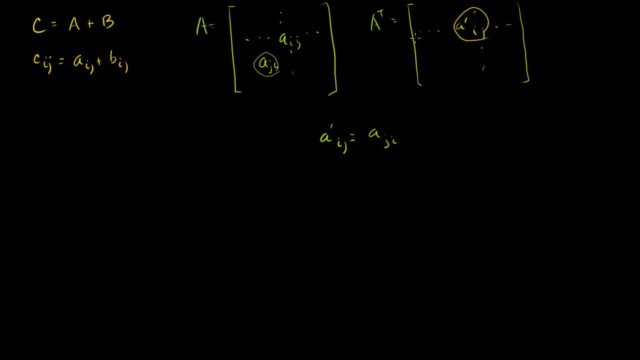 equal to this guy over here. if you switched the rows and columns, I think you can accept that And you can make the same argument for B. Let me actually draw it out. So if I make B, transpose the entry in the ith row and jth. 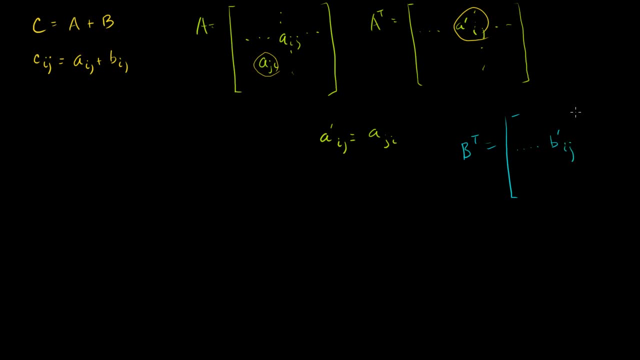 column. I'll call it B prime ij just like that, just like I did for A. So we could say that B prime ij is equal to you. take the matrix B, but it's going to be the entry. That's in the jth row and ith column. 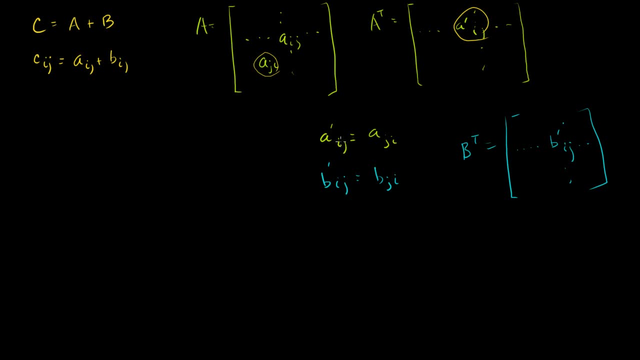 These are, you could almost say, the definition of the transpose. If I'm in the third row and second column now, it's going to be what was in the second row and third column. Fair enough, So what is so? we already have what Cij is equal to. 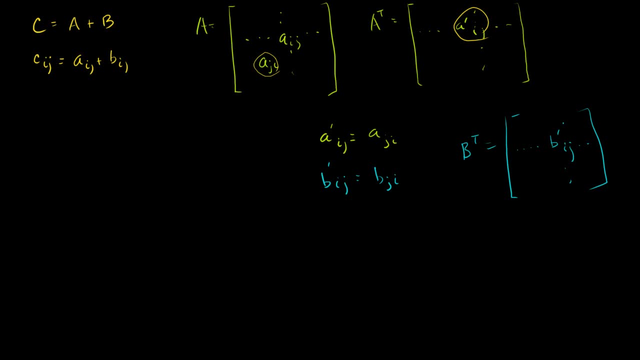 What's the transpose of Cij going to be equal to? Let me write that down So: C transpose. let me write it over here. Let me write C transpose. C transpose is equal to. I'll use the same notation. The prime means that we're taking entries in the. 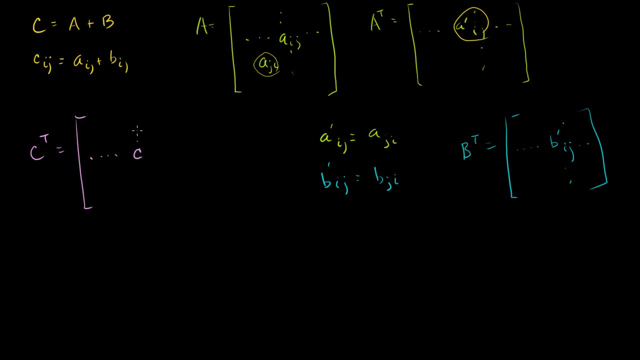 transpose. So C transpose is just going to be a bunch of entries ij. I'll put a little prime there showing that that's entries in the matrix of the transpose and not in C itself. And we know that C prime ij is equal to Cji. 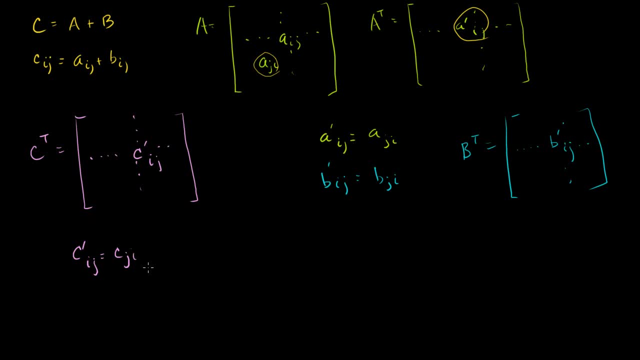 Nothing new at all. We've just expressed kind of the definition of the transpose for D. OK, These three matrices. Now what is Cji equal to? So let's focus on this a little bit. What is Cji equal to? 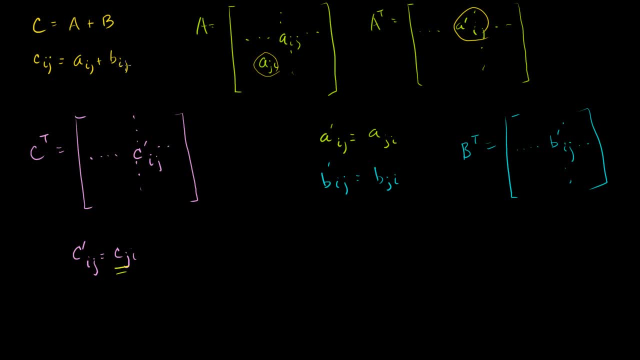 We know that Cij is equal to a sub ij plus b sub ij. So if you swap them around, this is going to be equal to You. just swap the j's and the i's: a sub ji plus b sub ji. I just used this information here. 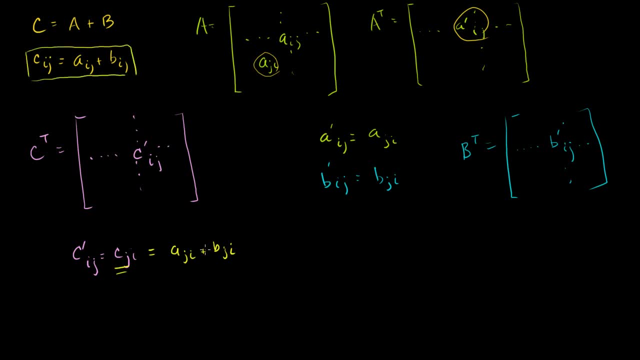 You could almost view it as this assumption or this definition. to go from this to this: If I had an x and a y here, I'd have an x and a y here and an x and a y here. I have a j and an i here, so I have a j and an i there. 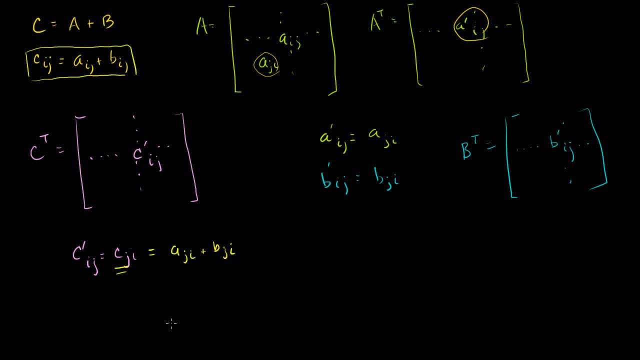 And a j and an i. right there. Now, what are these equal to? This is equal to this guy right here- is equal to the same entry for the transpose of A at ij, At ij, And this is equal to. This is equal to the same entry for the. 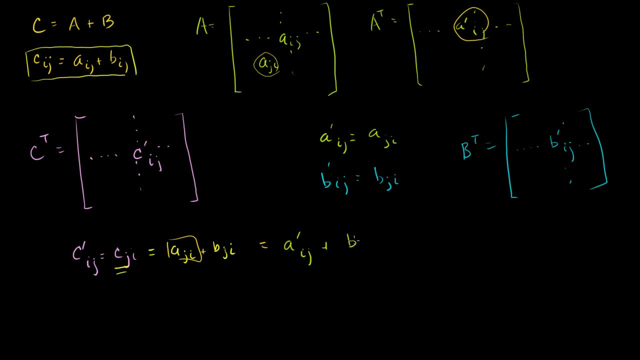 transpose of B at ij, The transpose at B at ij. Now, what is this telling us? It's telling us that the transpose of C, which is the same thing as A plus B, So it's saying that A plus B transpose. 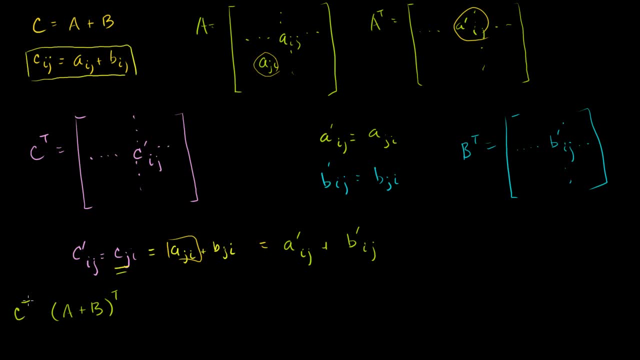 A plus B transpose is the same thing as C transpose. Let me write that C transpose is the same thing as A plus B transpose. So these are the entries And A plus B transpose right here. And what is this over here? What are these? 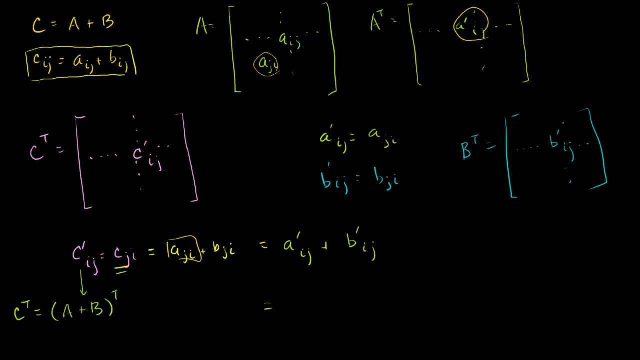 These are the entries right there. Let me do the equal sign over here. What are these? These are the entries in A- transpose plus B- transpose- Right, These are the entries in A- transpose. These are the entries in B- transpose. If you take the sum of the two, you're just adding up the. 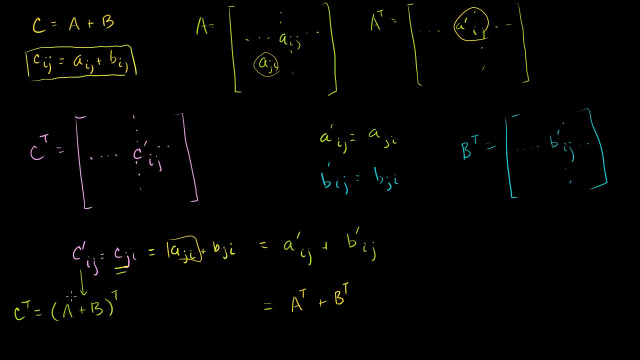 corresponding entries. So that's straightforward to show that if you take the sum of two matrices and then transpose it, it's equivalent to transposing them first and then taking their sum, which is a reasonably neat outcome. Let's do one more and I think we'll finish up all of our 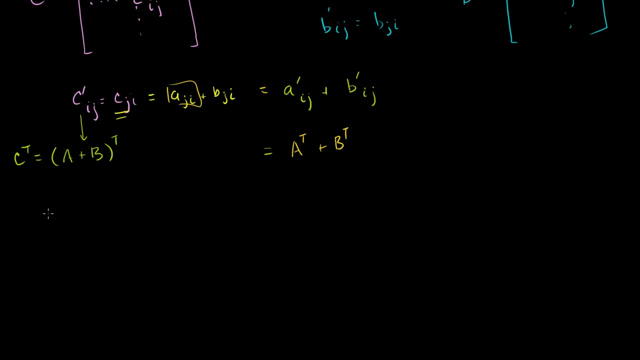 major transpose properties. Let's say that A inverse- This is going to be a slightly different take on things. We're still going to take the transpose. So if we know that A inverse is the inverse of A, that means that A times B. 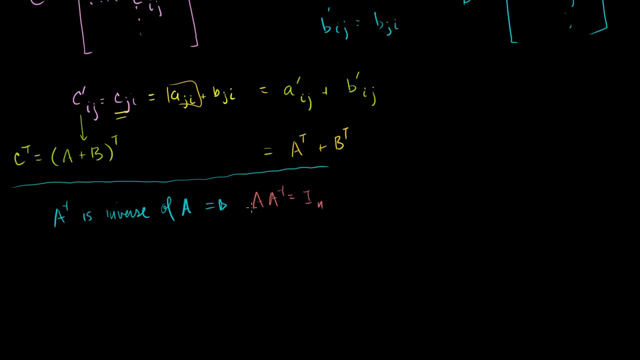 A inverse is equal to the identity matrix, assuming that these are n by n matrices, so it's the n-dimensional identity matrix and that A inverse times A is also going to be equal to the identity matrix. Now let's take the transpose of both sides of this equation. 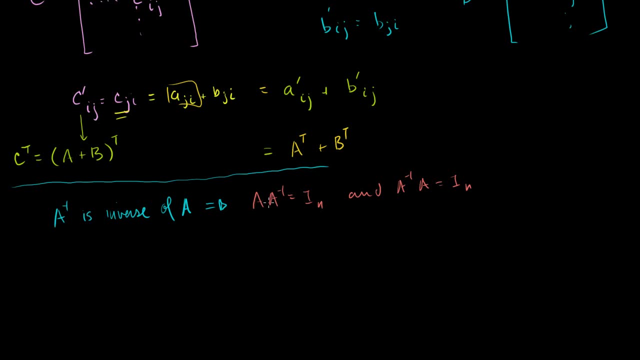 Let me start with. I'll do them both simultaneously. So if you take the transpose of both sides of the equation, you get A times A inverse Transpose. This is equal to the identity matrix transpose. Now, what's the transpose of the identity matrix? 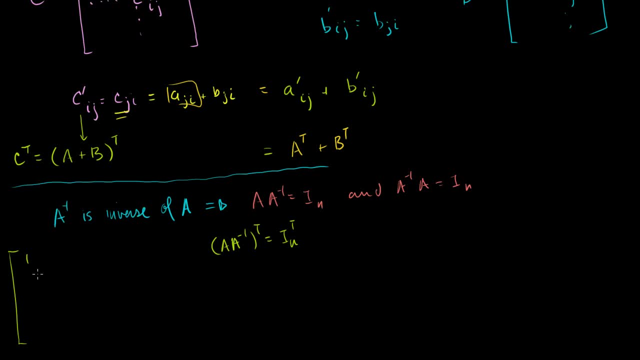 Let's draw it out. The identity matrix looks like this: You have just 1's all the way down the diagonal and everything else is 0. Everything else is 0. You could view this as I11,, I22, all the way down to INN. 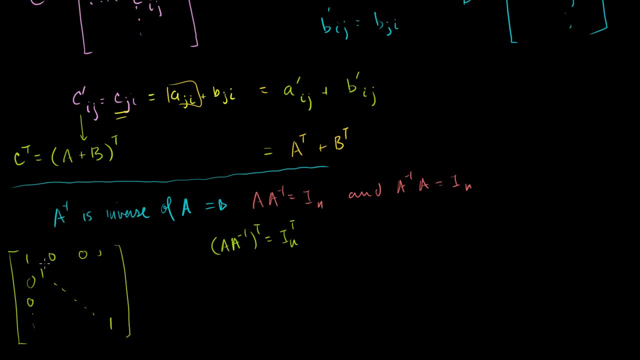 Everything else is 0. So when you take the transpose you're just swapping up the 0's. These guys don't change. The diagonal does not change when you take the transpose. So the transpose of the identity matrix is equal to the. 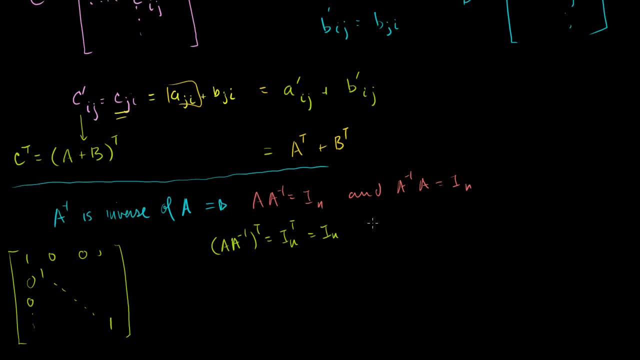 identity matrix, And so we can apply that same thing here. Let's take the transpose for this statement. So we know that A inverse times A transpose is equal to the identity matrix, transpose which is equal to the identity matrix, And then we know what happens when you take the transpose of.